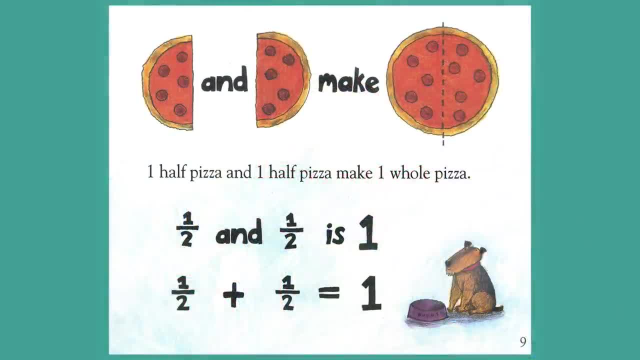 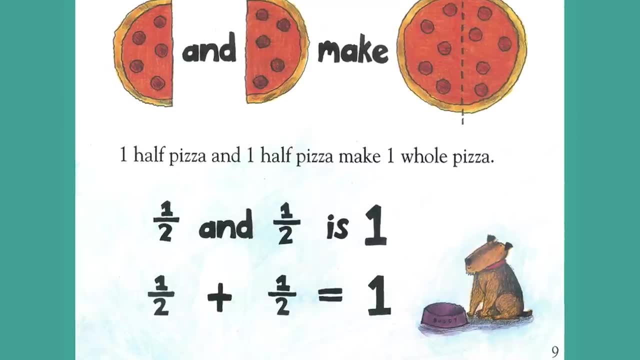 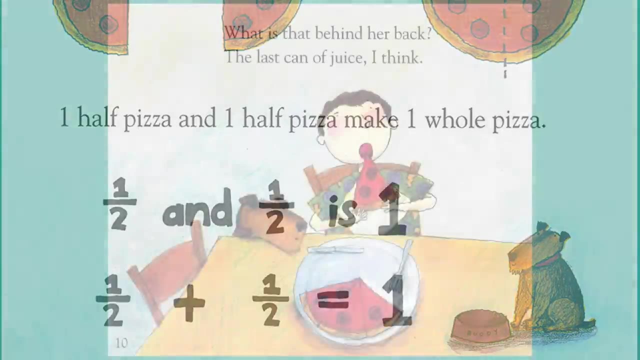 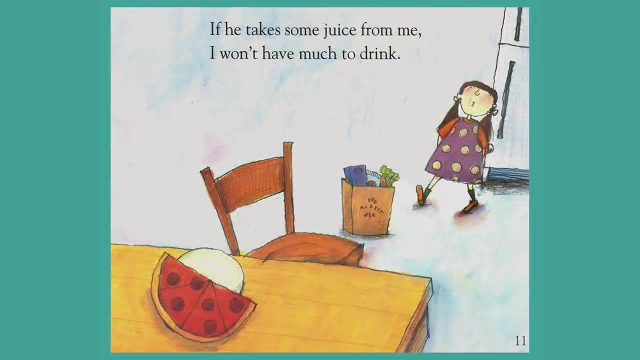 of you. One half pizza and one half pizza make one whole pizza. One half and one half is one. One half plus one half equals one. What is that behind her back? The last can of juice. I think If he takes some juice from me, I won't have much to drink. 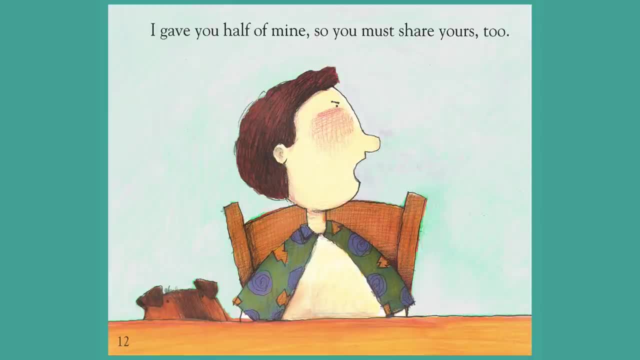 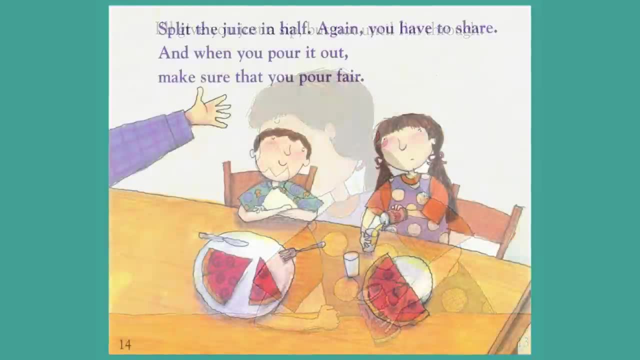 I gave you half of mine, so you must share yours too. I'll give you just a sip, but not until I'm through. Split the juice in half Again. you have to share Now. you have to share only half, and when you pour it out, make sure that you pour fair. 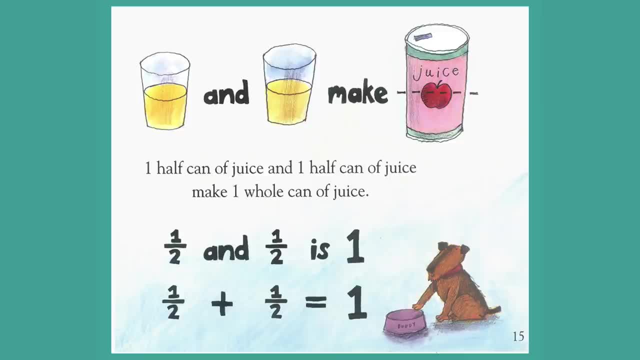 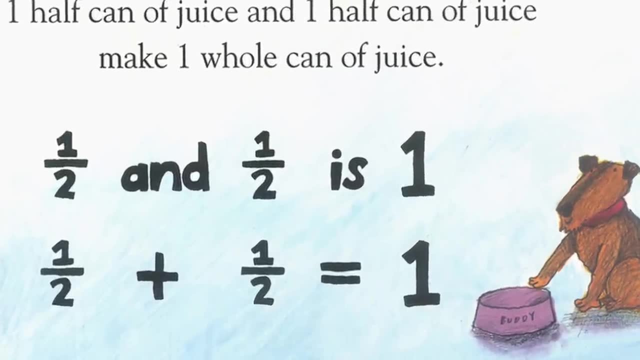 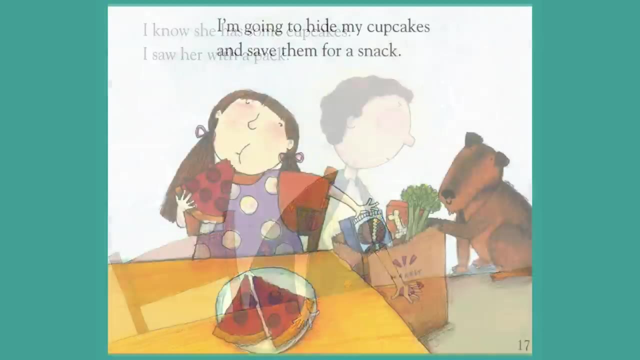 One half can of juice and one half can of juice make one whole can of juice. One half and one half is one. One half plus one half equals one. I know she has some cupcakes. I saw her with a pack. I'm going to hide my cupcakes and save them. 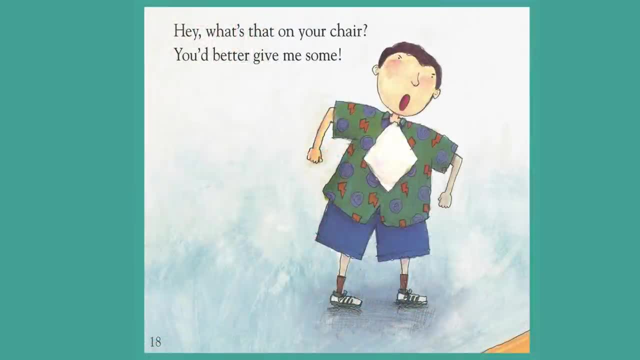 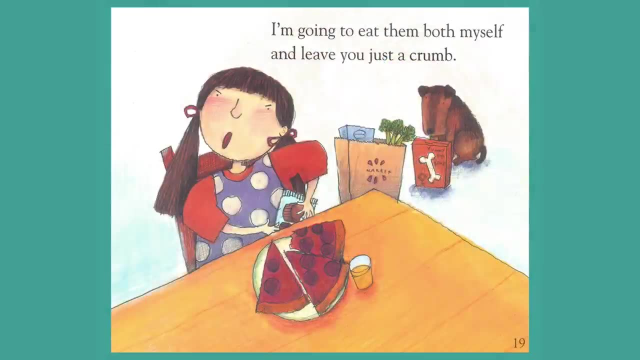 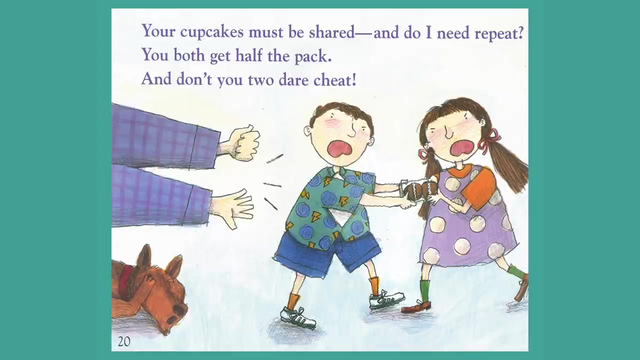 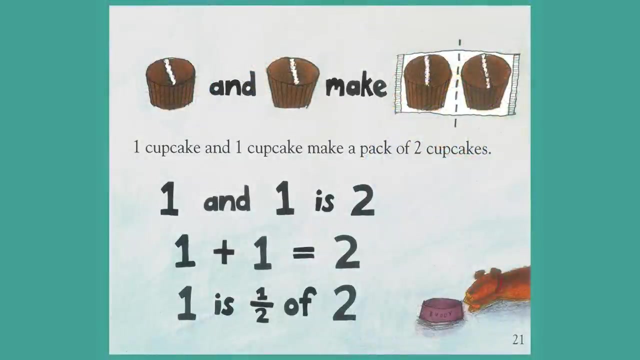 save them for a snack. Hey, what's that on your chair? You'd better give me some. I'm going to eat them both myself and leave you just a crumb. Your cupcakes must be shared, and do I need repeat? You both get half the pack, and don't you two dare cheat? One cupcake and one cupcake. 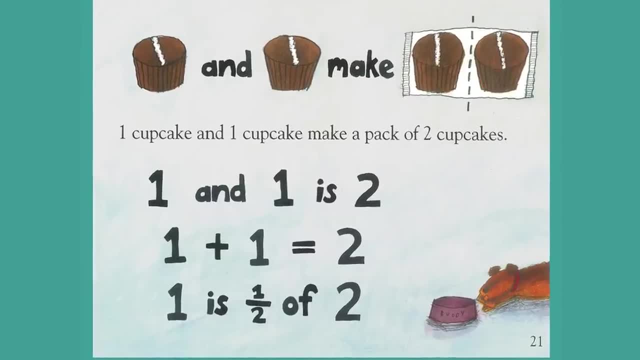 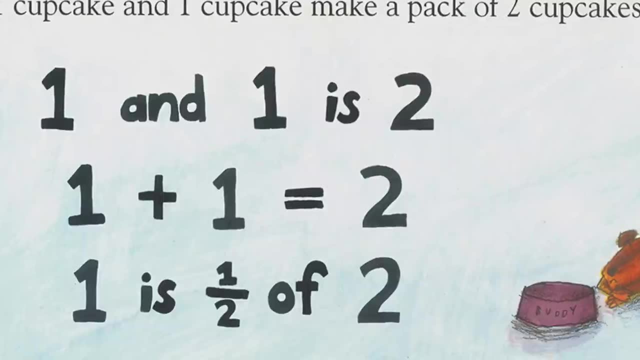 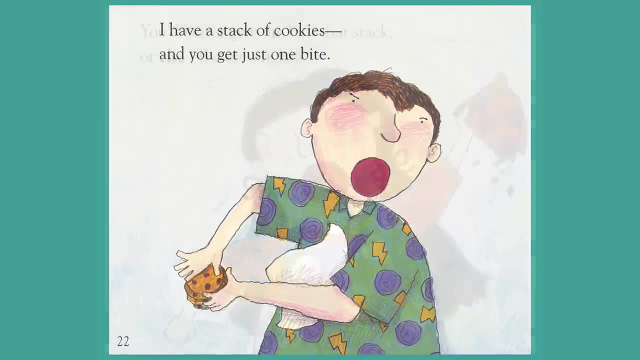 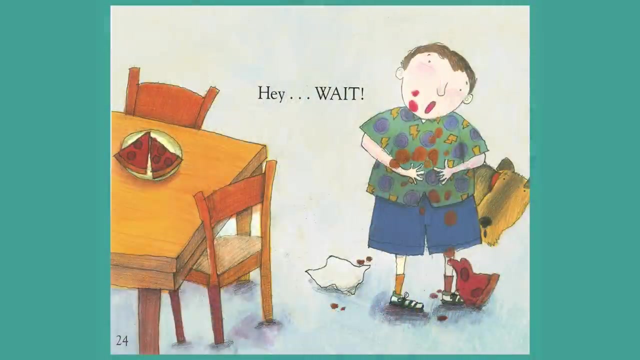 make a pack of two cupcakes. One and one is two. One plus one equals two, One is one-half of two. I have a stack of cookies and you get just one bite. You'd better give me half that stack, or else I'll start a fight. Hey, wait Too late. Food fight. 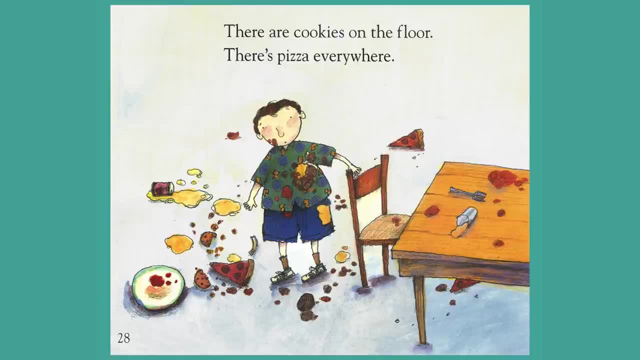 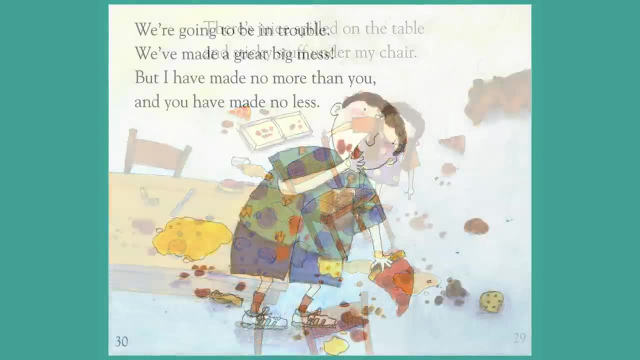 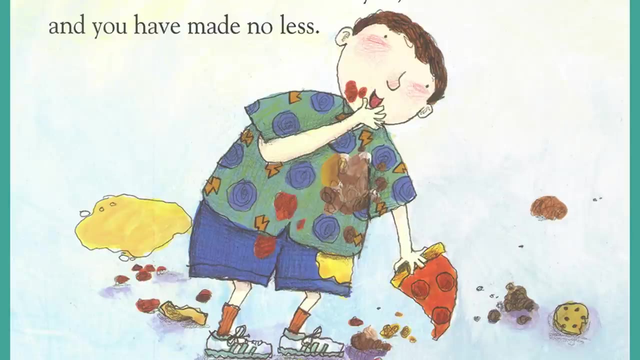 There are cookies on the floor, There's pizza everywhere, There's juice spilled on the table and sticky stuff under my chair. We're going to be in trouble. We've made a great big mess, But I have made no more than you and you have made no less. We'd better each.